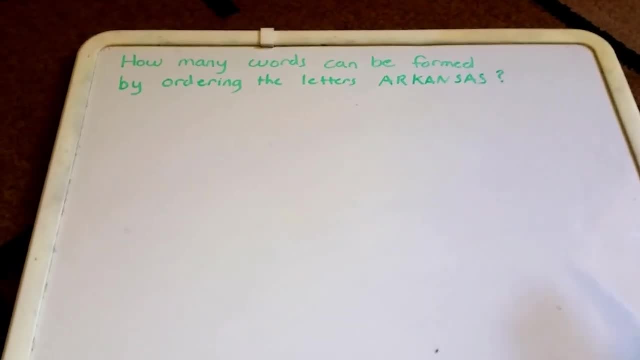 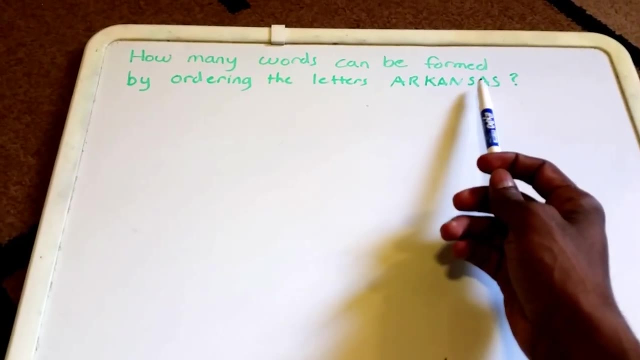 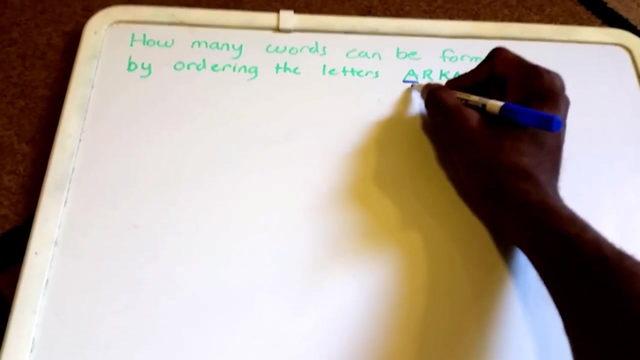 Hey guys and welcome to this video. So in this video we want to see how many words can be formed by ordering the letters A-R-K-A-N-S-A-S, which is the word Arkansas. So the first thing we need to do to get started is count how many letters we have in total, or spots, which would be 1,, 2,, 3,. 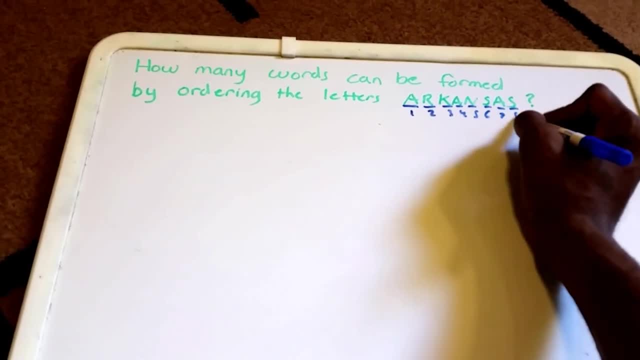 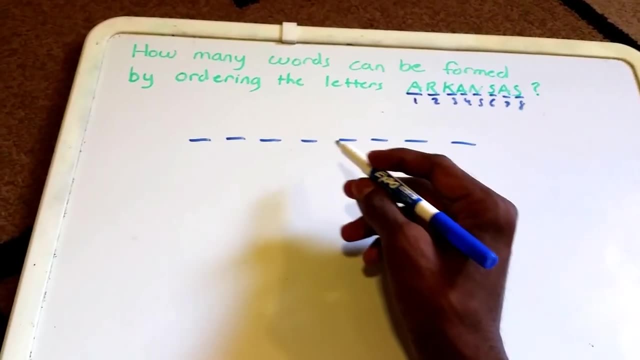 4, 5,, 6, 7,, 8 different spots. So I'm going to rewrite that here: 1, 2, 3, 4, 5, 6,, 7, 8. so we have 8 different spots, and first thing we need to do is figure out how we want to place the 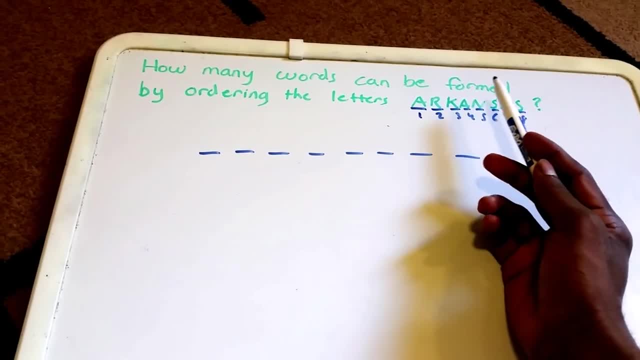 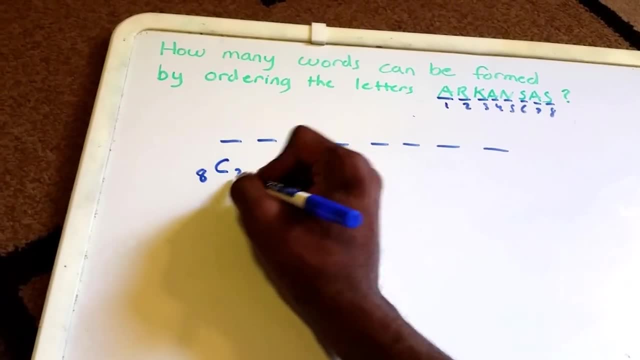 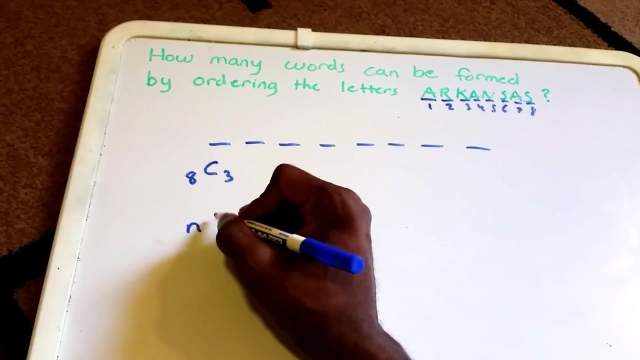 3 A's in any 3 of the 8 positions. So we could do that using this notation, which is 8C3. and for those of you that don't know, this is the combination formula, and the combination formula- I will write it right down here- is NCK, or written like that, or maybe you might see it as a NK or. 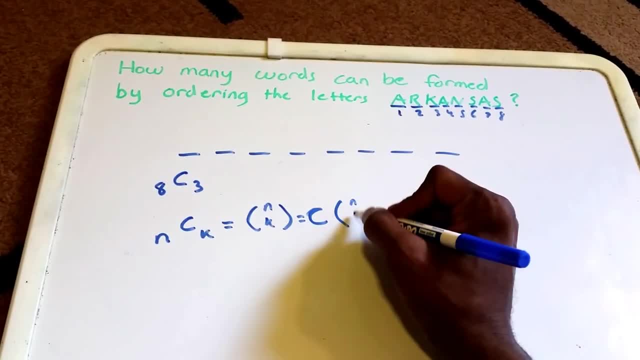 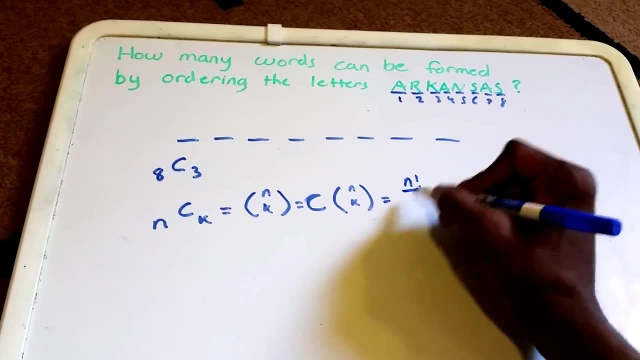 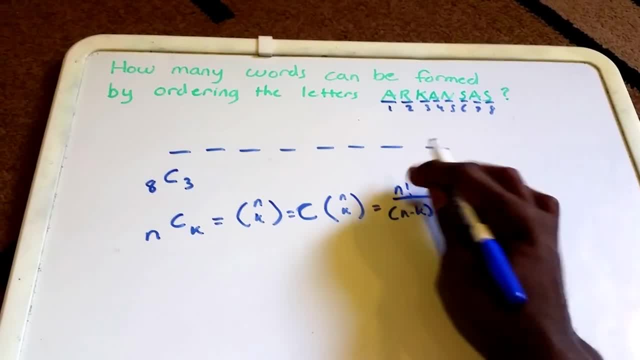 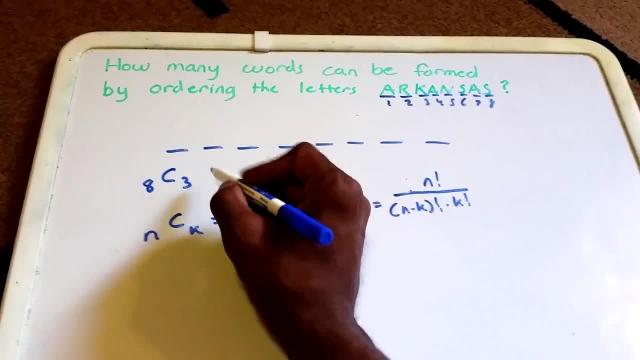 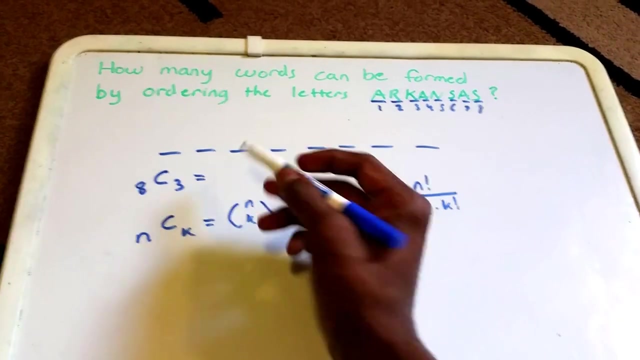 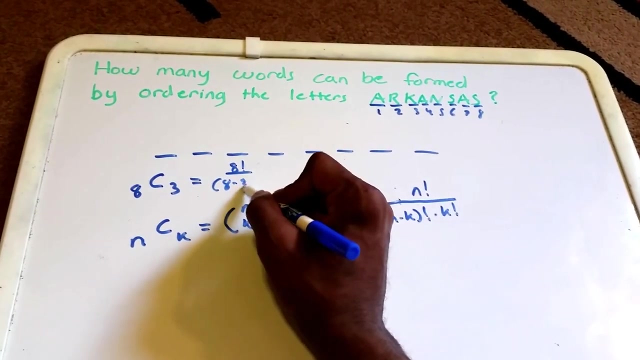 K factorial, so all that's over N factorial, just like that. Alright. so using this same formula here, what we get with 8C3, which is saying that we have a total of 8C3 and we have a total of 8 spots and we want to choose 3 of them, we get 8 factorial over 8, minus 3 factorial times 3. 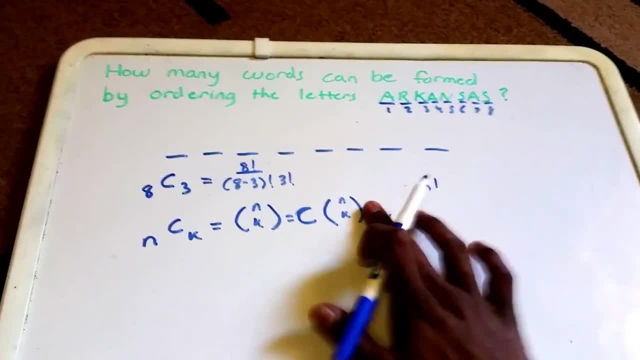 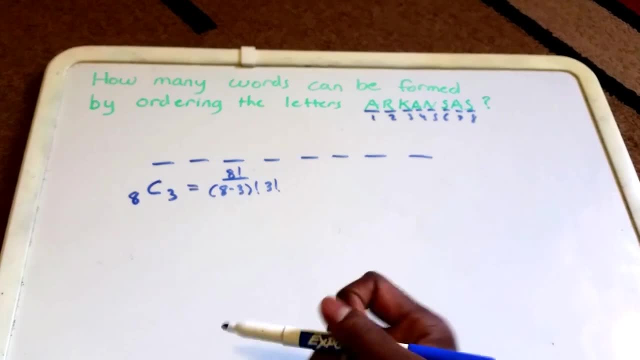 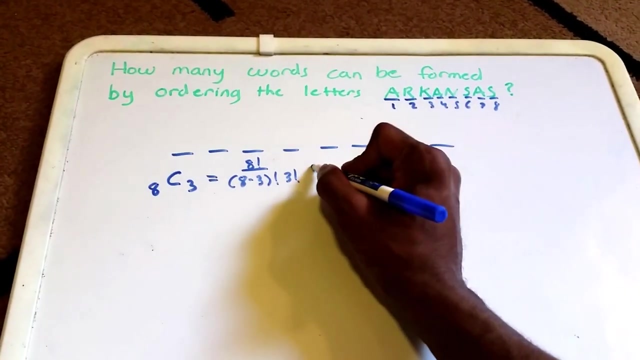 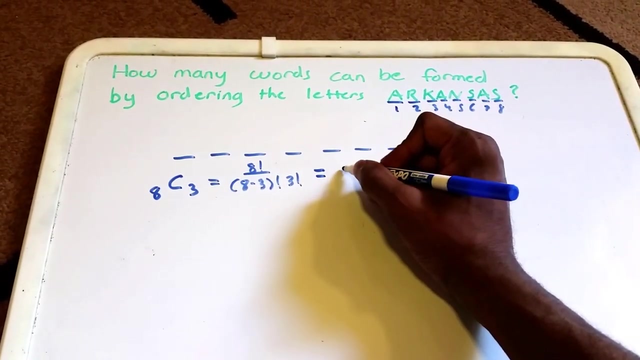 factorial. Alright, so I'm going to erase the formula here. Perfect. So this is how we can place the 3 A's in any 3 of the 8 positions. So let me finish out, try to simplify it. so this is just 8 times 7, which is 56, and make sure you put that there. 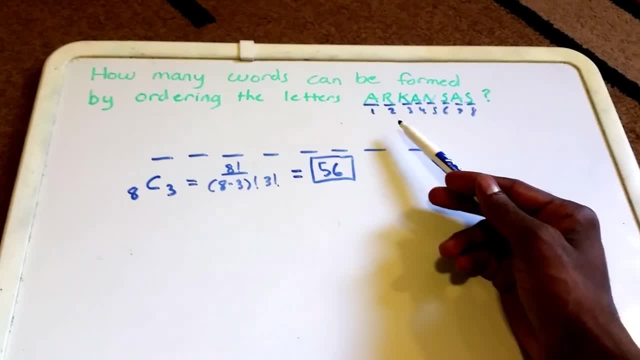 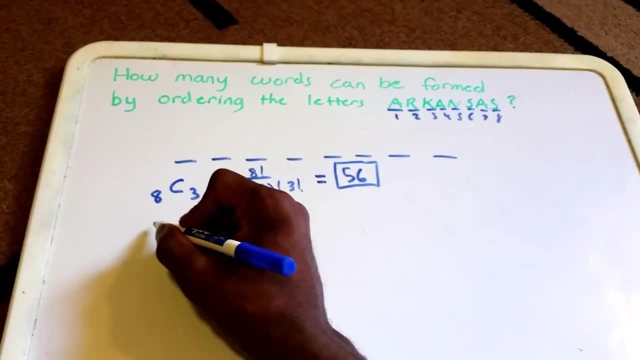 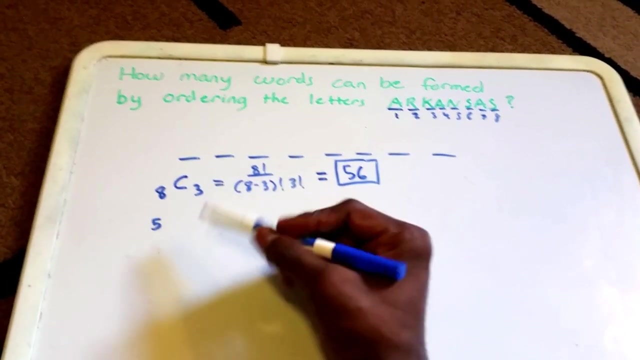 alright. so next up, I'm looking to see. I'm looking at these S's, because they are the next letters that appear the most, and so we have 5 spots left, because we chose 3 of them already. so now we have 8 minus 3, which is 5. 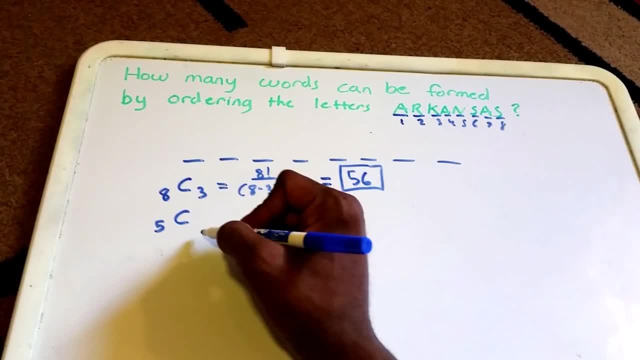 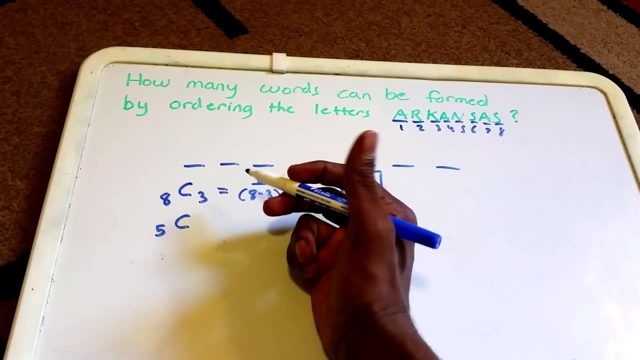 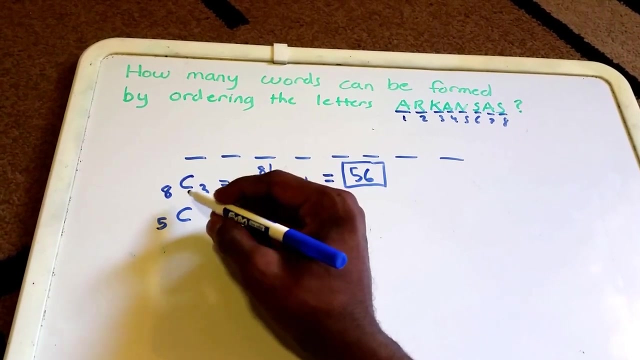 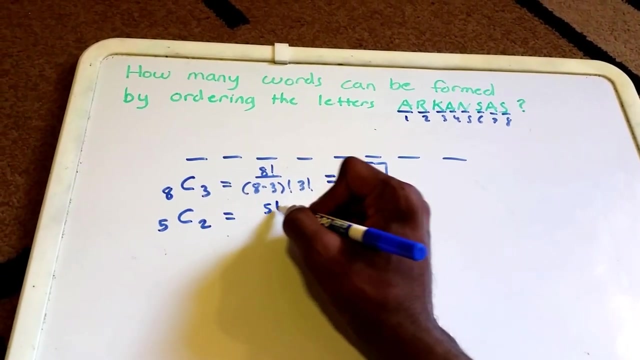 and we want to see how we can place any two of the S's in any two of the remaining positions or place the 2 S's in any two of the remaining 5 positions. So that is 5, we're choosing 2. and so that can be written as 5 factorial over 5 minus 2 factorial. 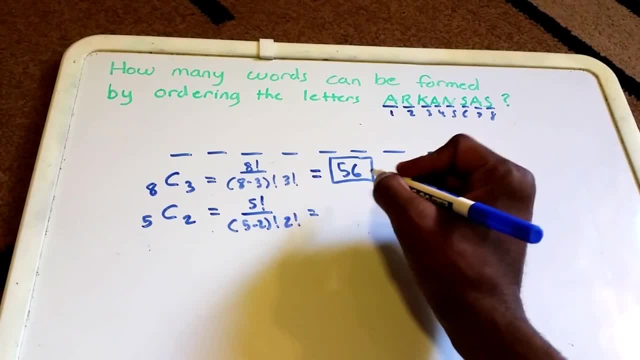 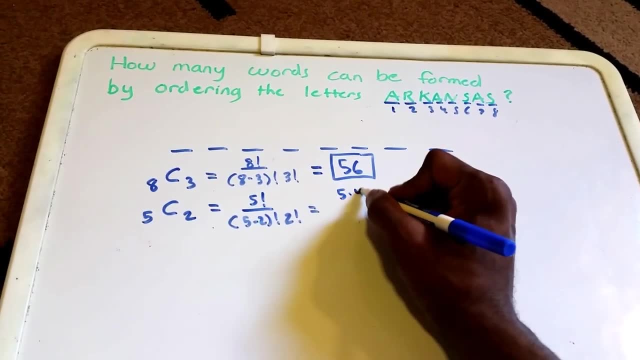 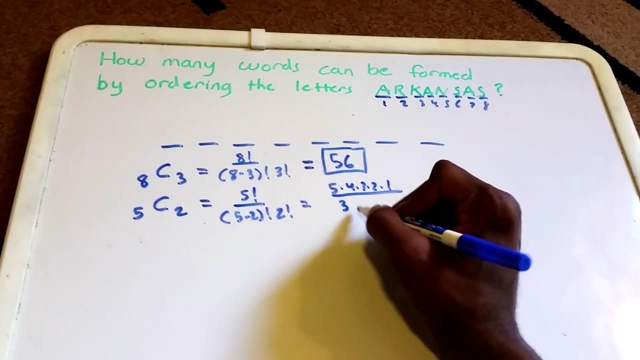 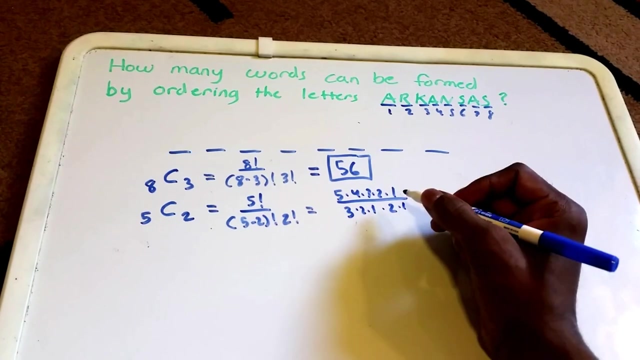 times 2, factorial. factorial, which is equal to: let's see this: I'm gonna have to write out a little bit: 5 times 4 times 3 times 2 times 1, over 3 times 2 times 1 times 2 times 1. okay, so this will give me. let's see, this will cross out here. so this is. 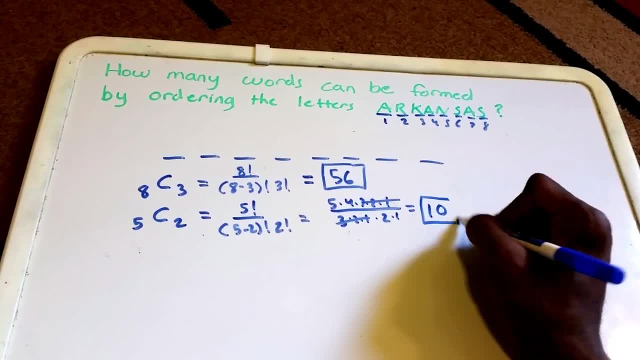 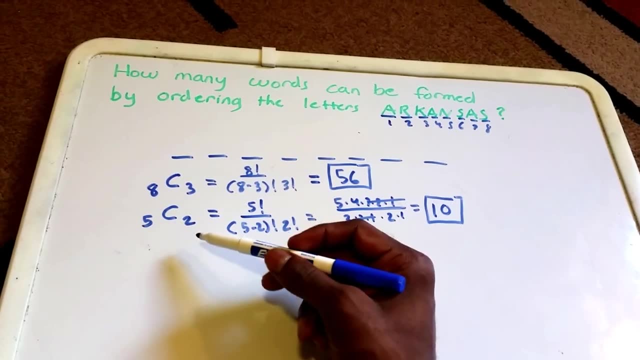 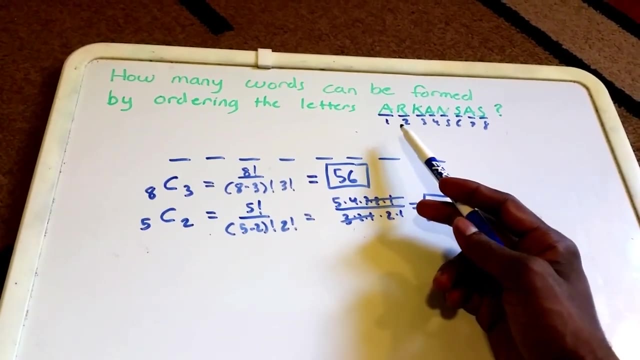 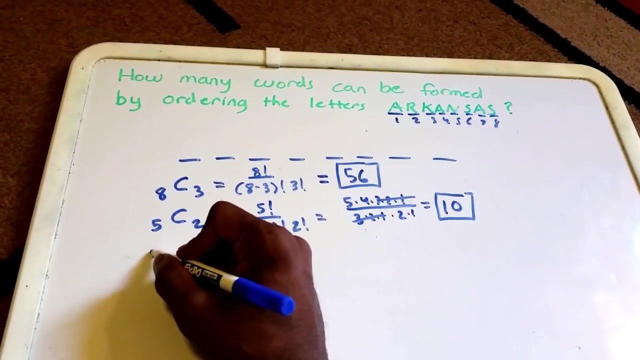 like this will give me 5 times 2, which is 10. okay, so now we have chosen five spots already, so that leaves us with three left. so let's take a look at the R and let's place the R in any one of the remaining three positions. so we have. 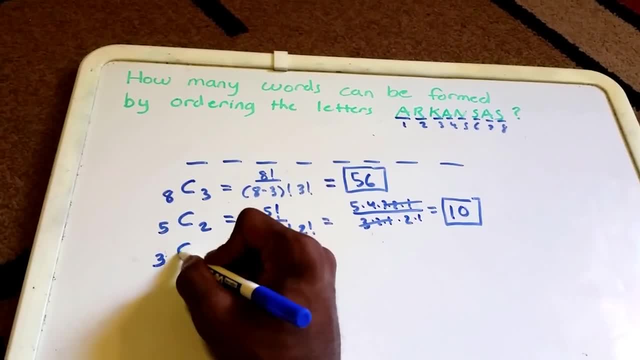 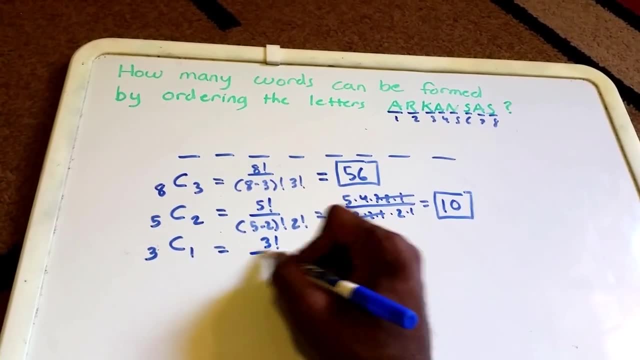 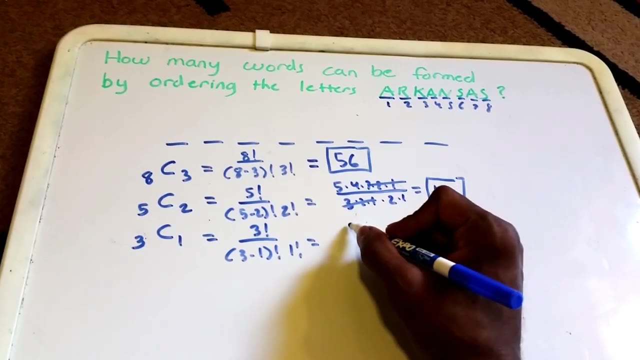 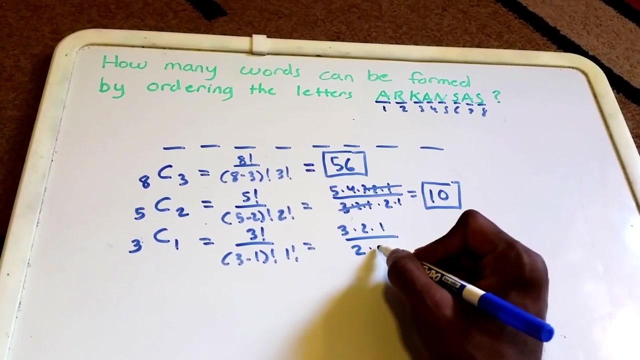 three positions left and we want to choose you one. R, so this is equal to 3 factorial over 3 minus 1 factorial times 1 factorial, which is equal to 3 times 2 times 1 over 2 times 1, which is equal to.